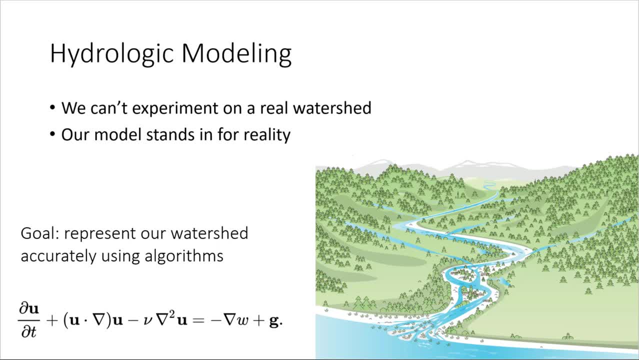 We can't have a side-by-side comparison of a control and an experiment. In order to experiment on a watershed, we need to use a model as a stand-in for the real thing. Instead of soil and plants, we have equations that govern how much water goes where. 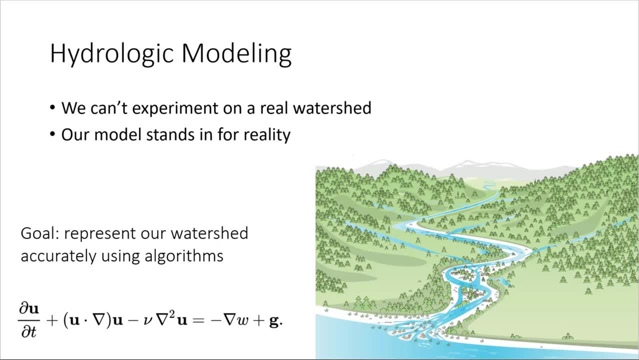 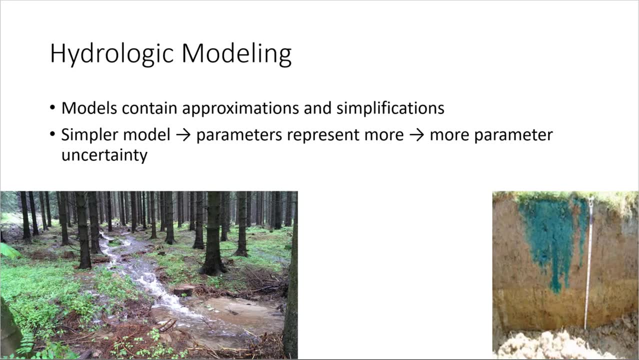 These equations represent the physical world in a deterministic way. It is necessary for a model of something as complex as the flow of water through the environment to contain approximations and simplifications of the real world, Even if we could represent the entire watershed at the atomic level. 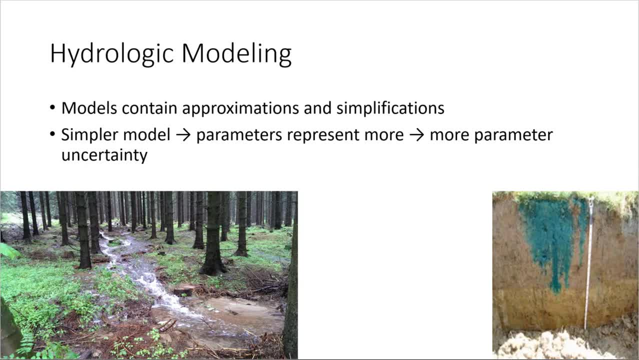 the measurement of the physical properties of the watershed necessary to model all the physics would contain uncertainty. Then applying the physics at that scale would be computationally prohibitive. Models should be as simple of a representation of the system being modeled as needed to answer the question or perform the experiment. 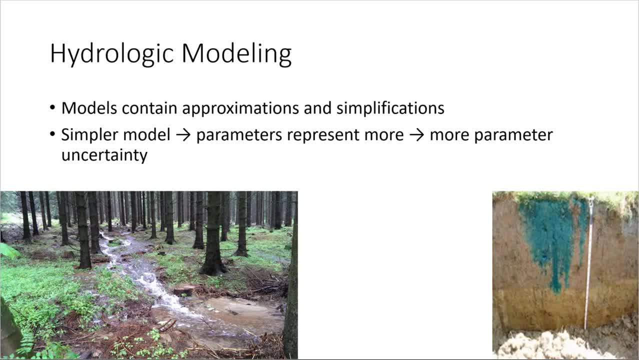 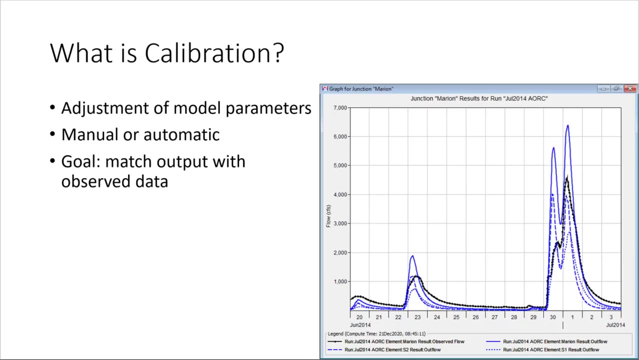 When several related processes are rolled into one algorithm to represent them, the parameters of that algorithm become more and more abstract and uncertain. While the parameters become more uncertain, their level of abstraction also lends them well to being determined empirically. Our hydrologic model is a collection of parametric algorithms that simulate the hydrologic cycle. 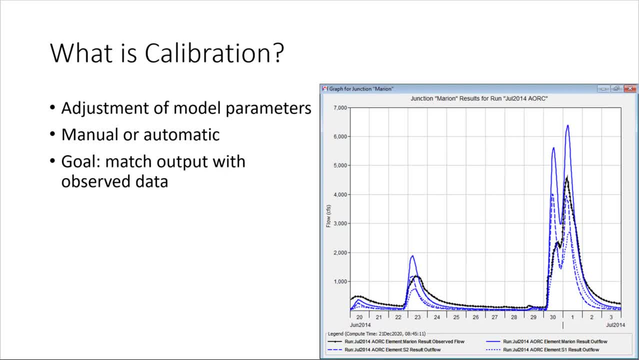 It is up to us as modelers to determine what the appropriate parameters for those algorithms are. We want to make our algorithmic representation of the watershed match the actual watershed across a wide range of conditions. Usually, we determine if our model matches reality by comparing model output for observed past events. 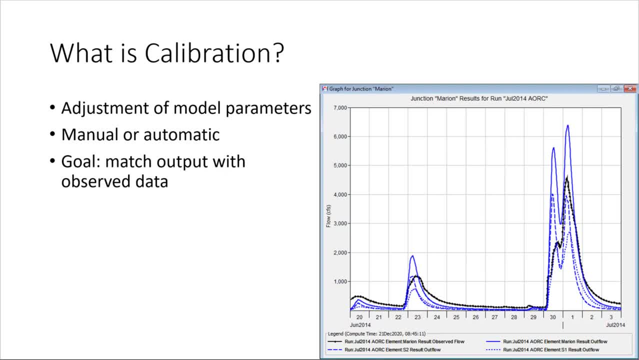 and seeing if key results match, We may consider whether the simulation of streamflow at locations where we have flow observations match reasonably well. We may also compare observations for other hydrologic processes such as snowmelt and accumulation and evapotranspiration. 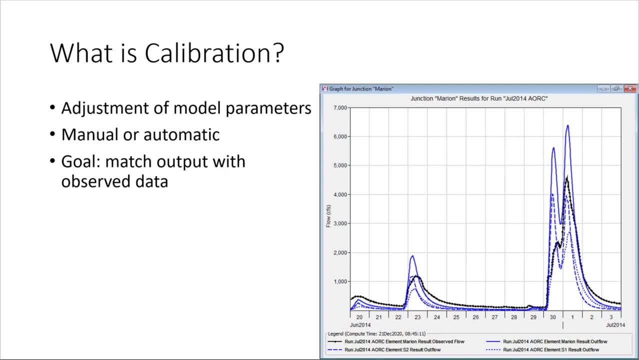 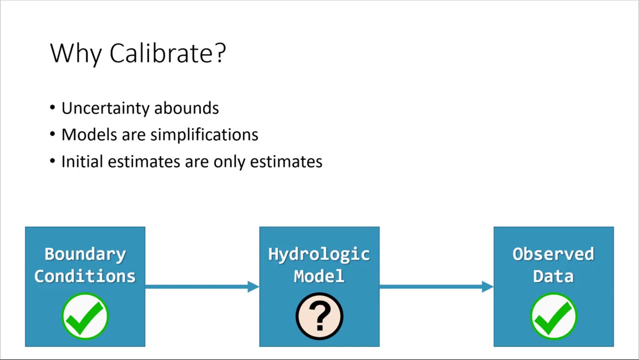 There are some so-called automated tools for performing calibration, but the most reliable way to produce a calibrated model with reasonable parameters is to change the parameters yourself until the model results match observed data. There is uncertainty inherent in all parts of the hydrologic modeling process. 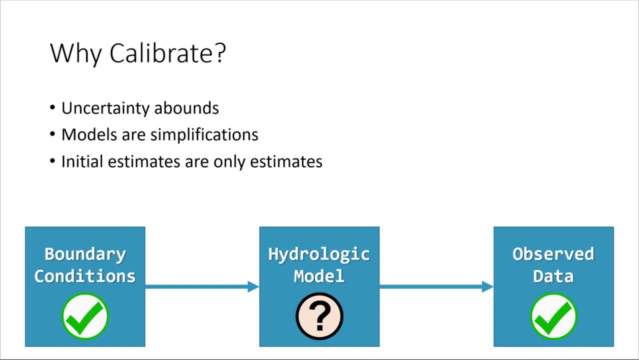 The data used to define the model has measurement error: everything from elevation data and land use data to meteorologic and hydrologic boundary conditions. Process simplifications can create parameters that represent several things all rolled into one number. Models are also abstractions of the real world. 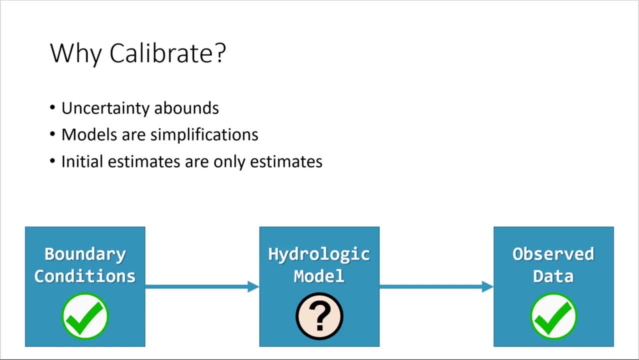 Even the most detailed physical models are simplifications of the hydrologic cycle. When we make an initial estimate of a parameter from physical data, it is just that an estimate Using the same technique across many watersheds will, on average, get you close to a good value. 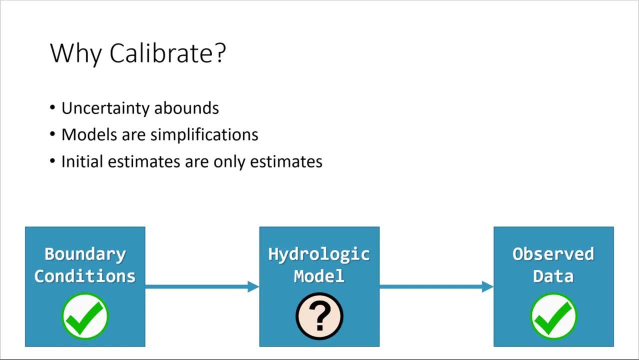 but each individual estimate may be off. We assume that any mismatch between the hydrologic results and the observed data are due to misspecification of hydrologic model parameters. There are more advanced techniques involved in jointly assessing uncertainty in boundary conditions, hydrologic model parameters and the observed data, but that's out of scope here. 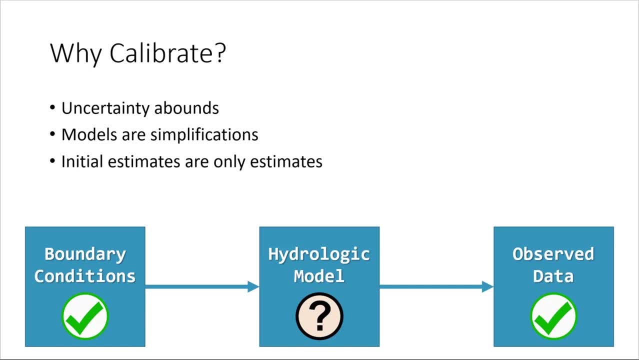 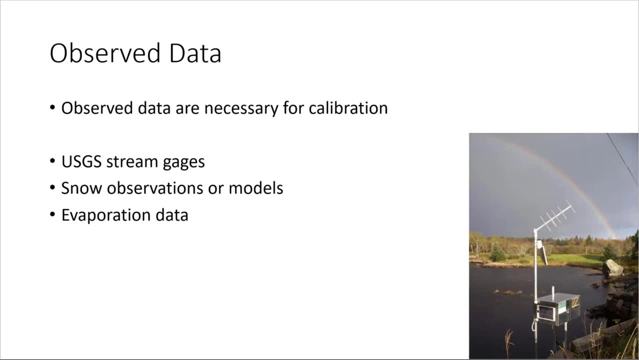 What we want in the end is a model that represents our watershed well, even when we change the boundary conditions out from underneath it. Observed data are the key to knowing if our model represents reality or not. A known standard that we can compare the model to will give us an assessment of its performance. 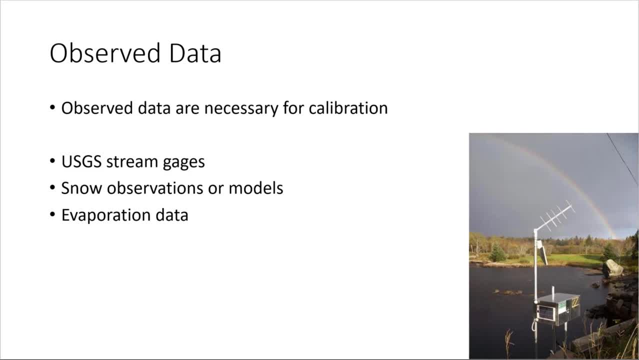 Usually we are interested in calibrating flow, so we reach for instantaneous data. We can use streamflow data when we can. Occasionally only coarse time-step data, such as daily average data, are available, and we can aim for that instead. 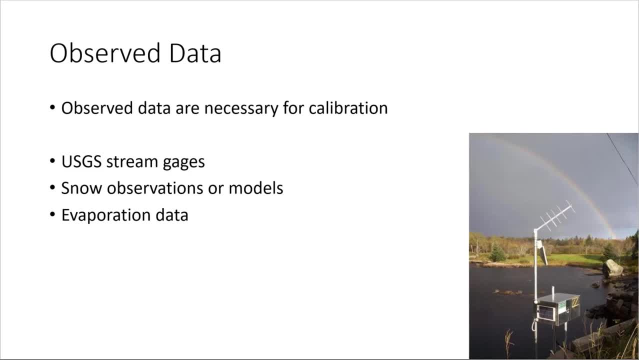 Other times the processes are more complicated. In snow-dominant watersheds, we may want to calibrate the snow processes independently, using observed or modeled snow data. For continuous calibration, it might be beneficial to calibrate the evapotranspiration process. 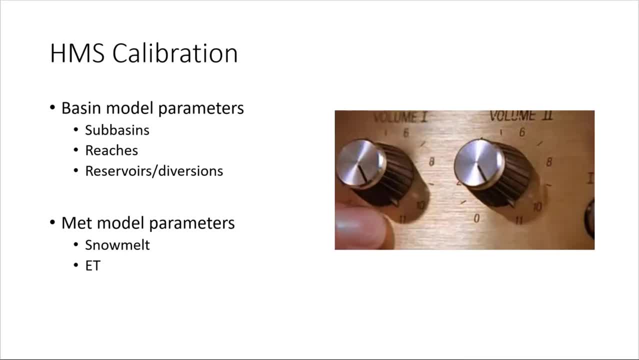 although data to do so may be rare. When calibrating an HEC-HMS model, we are changing the parameter values to the processes inside the basin model and the meteorologic model. In the basin model, the primary location we will make adjustments is in the subbasin elements. 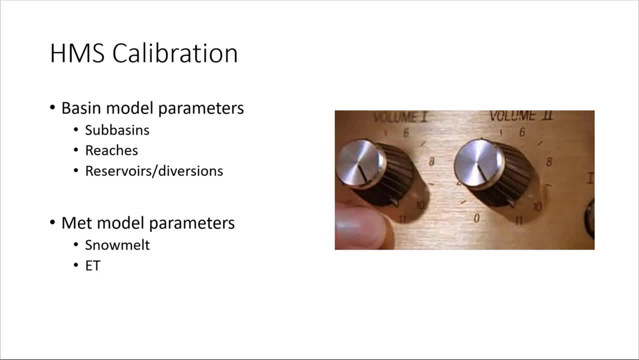 They handle the majority of the rainfall runoff process. For more complicated watersheds, where elements are connected with reaches, we may adjust reach parameters to get channel routing correct. In order to model historical events correctly, we may also need to make changes to reservoir or diversion operations. 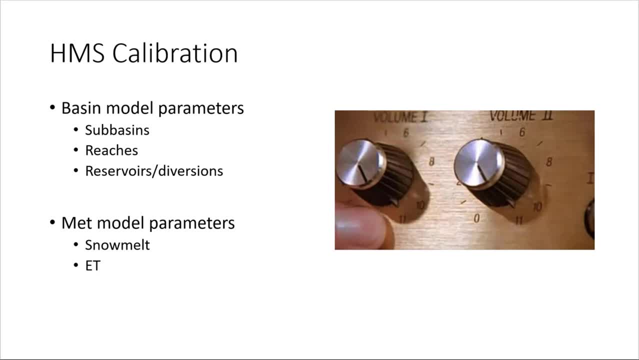 Within the MET model, the most common changes are to snowmelt parameters and watersheds that need it. The temperature index method has several tunable parameters that can improve model performance, not only in the explicit snowmelt and accumulation processes, but also in the resulting runoff. 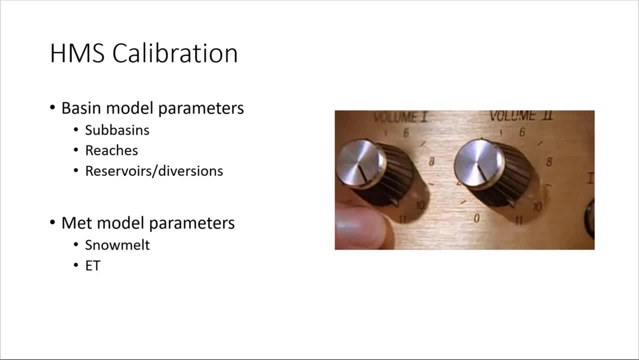 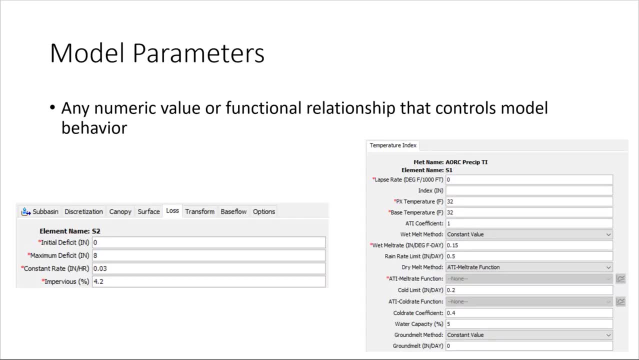 ET may be adjusted in a fine sense to match observations or, more coarsely, to address mismatches in overall discharge volume. Some model parameters are typically treated as fixed, while others are allowed to freely vary during the calibration process. For example, the subbasin element is a model parameter. 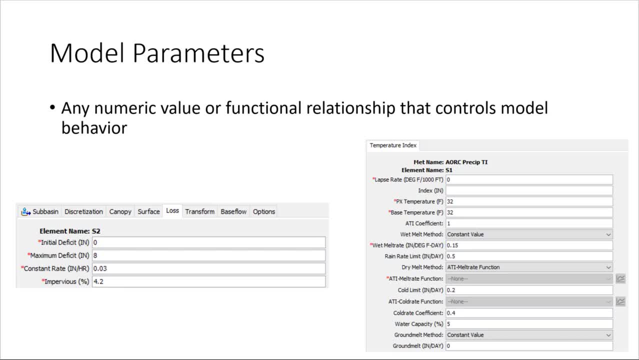 but it isn't changed. while calibrating On the left is a subbasin element and the parameters for the loss process are shown, The user is selected the deficit and constant loss method as the most appropriate method for modeling the loss process in this watershed. 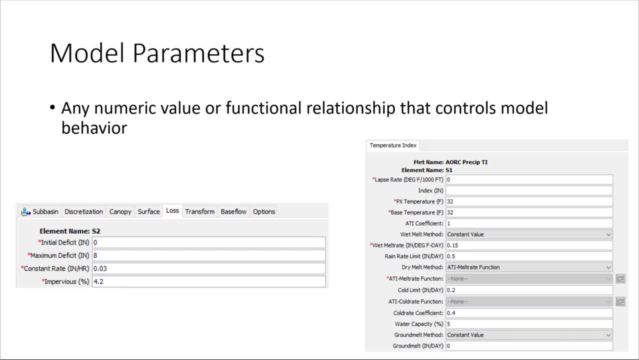 The method is not initially parameterized with any values and it is up to the user to provide initial estimates for those parameter values. Then, during the calibration process, these values are adjusted in order to improve model performance. On the right side is the subbasin element. 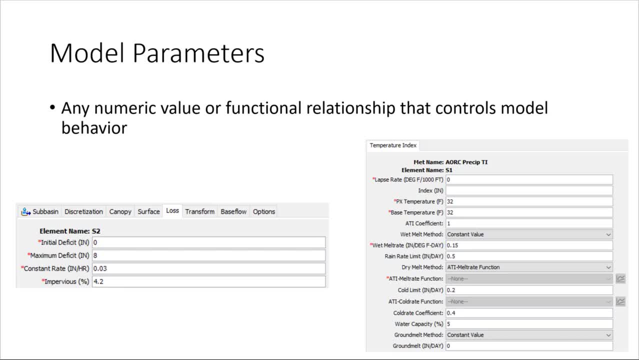 and this is the subbasin settings for the temperature index snow model. This is a highly parameterized model process and can include more than single numeric value parameters. ATI melt rate functions and ATI cold rate functions are an empirical representation of a mathematical function and can be calibrated to improve model performance. 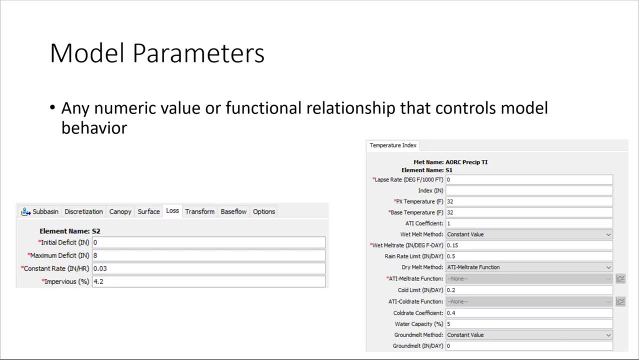 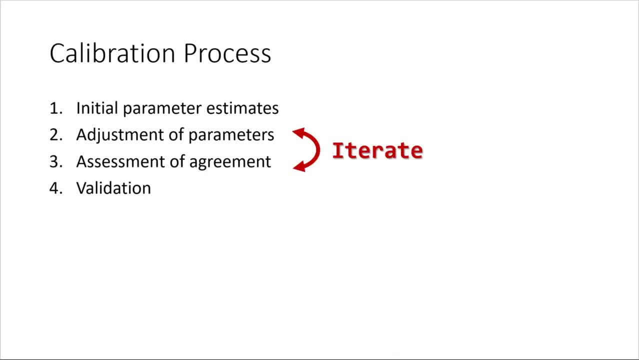 It is again up to the user to initially parameterize the model with parameter values and then to adjust those parameters to improve model performance. There is a four-step process to calibrating a hydrologic model. First, you must determine a set of initial parameters. 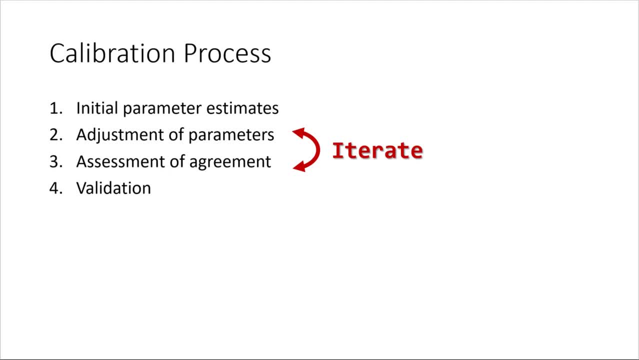 to get the model to run and to assess the initial performance of the model. There are helpful tools for getting useful parameters based on data about the watershed. Next, you will begin to adjust the model parameters so that the agreement between the model and the observed data begins to improve. 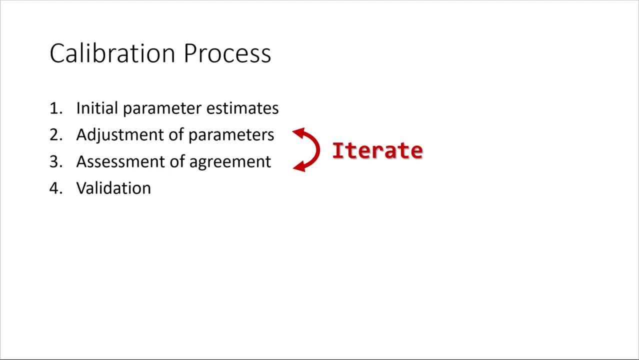 With each change in parameters, take the time to assess how the model performance changes, Then go back to the parameter adjustment and iterate. You will loop between step 2 and 3 many times, even if the initial parameter estimates aren't bad. 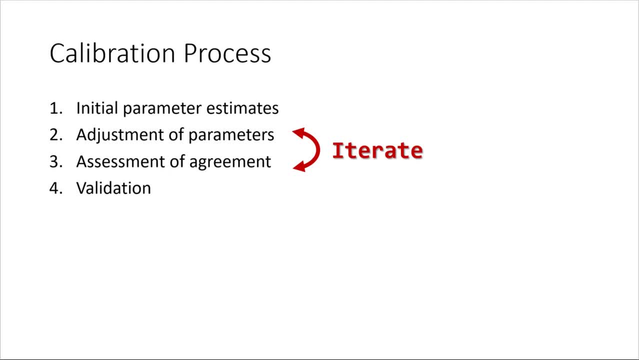 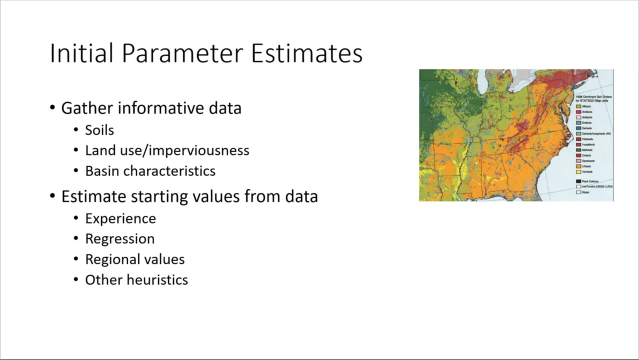 Finally, once you have a candidate set of calibration parameters, you will run a validation simulation which helps ensure your parameters are useful outside of the event you used for calibration. HMS does not provide default values for model parameters. It is up to the user to provide reasonable starting values. 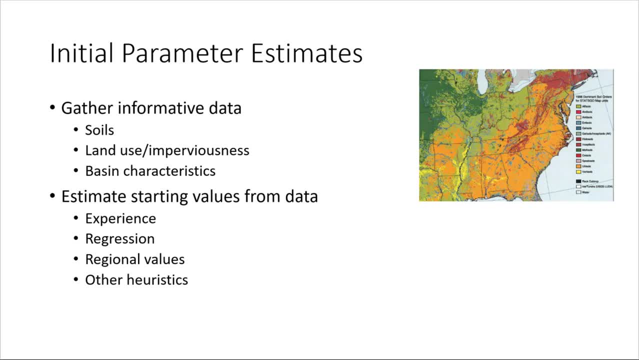 Experienced modelers can draw in knowledge of similar models to choose reasonable starting parameters. Models for similar watersheds may have similar parameters and parameter values from previous model calibrations may provide good starting points. Data-driven approaches use physical information to estimate model parameter values. 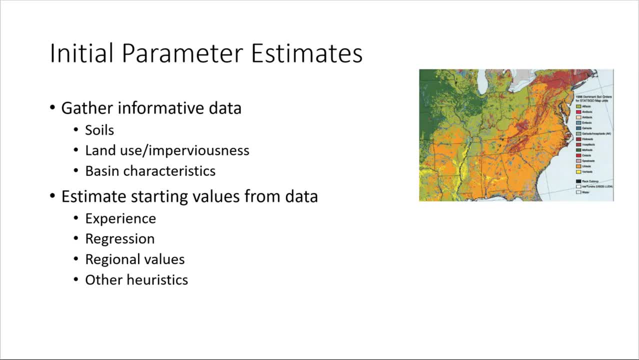 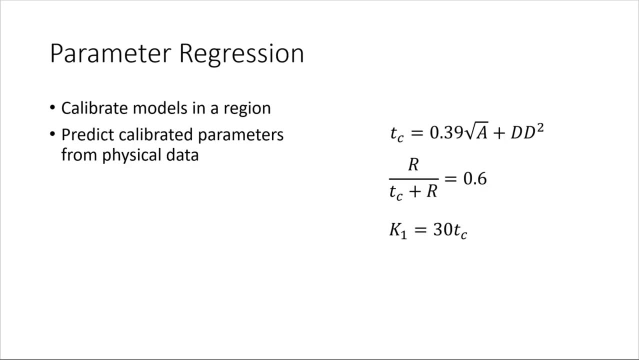 Typically, these estimates are driven by data such as soil surveys, land use, land cover and imperviousness, data basin, physical characteristics and so on. Regression equations are sometimes developed from regional studies. Several models are calibrated and their physical properties retained. 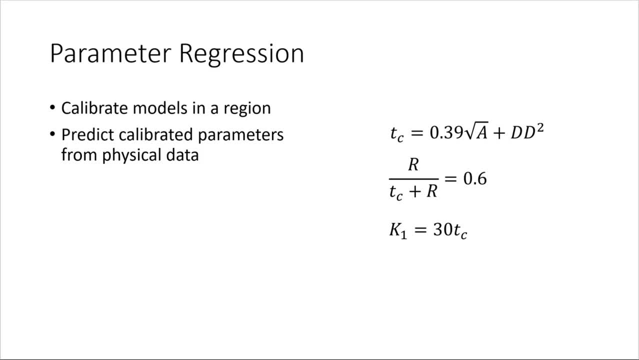 Then a regression model is fit to the data so that the physical properties explain the variability in the calibrated parameters. These equations can then be used to estimate parameters in other watersheds. An example of a predictor equation for time of concentration based on drainage area and drainage density is shown on the right. 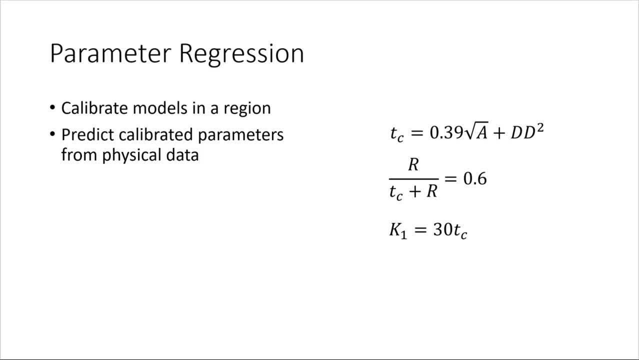 Time of concentration tends to be easier to predict using regional regression than some other parameters are. Over time modelers have developed other useful guidelines for estimating starting parameters. Some parameters are easier to estimate from physical data, such as constant loss rate, percent impervious time of concentration and so on. 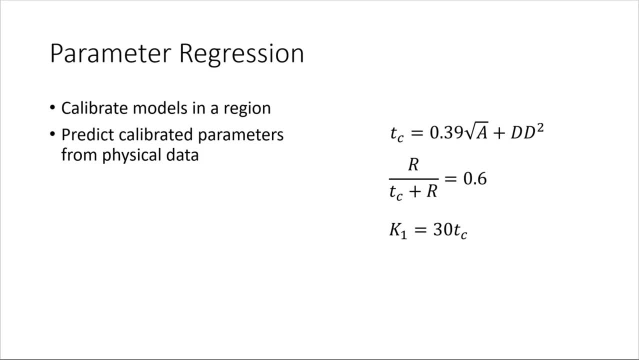 Then simple rules can be applied to these estimated parameter values to estimate other parameter values. Two examples of this are shown in the lower right. After estimating time of concentration, the storage coefficient can be estimated using an empirical relationship such as this: Typical values for this ratio are in the range of 0.5 to 0.8.. 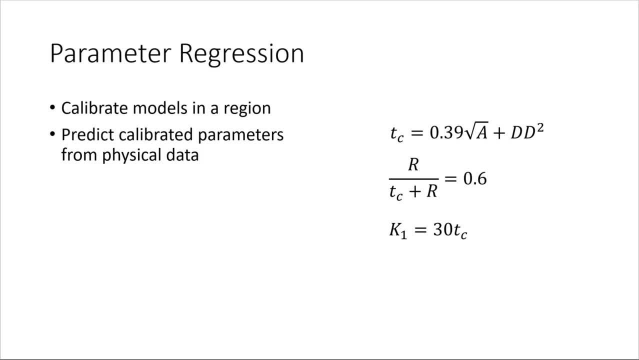 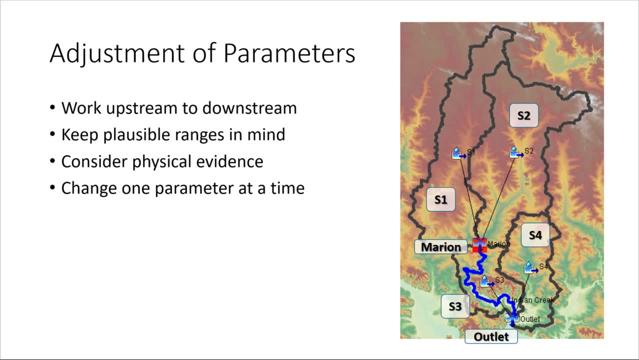 For linear reservoir groundwater parameters, the fast response layer coefficient can initially be estimated by 30 times the time of concentration. Here are some simple rules for a successful calibration. First, work upstream to downstream. Get a small area performing well and then move downstream. 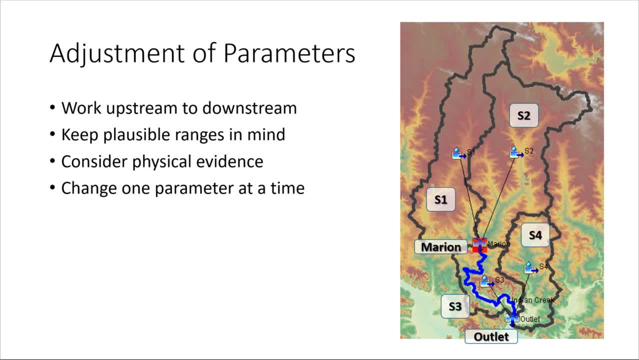 and leave the smaller areas alone when adjusting parameters further downstream. In the image shown, you would calibrate S1 and S2 above the Marion Junction first and then calibrate S3, S4, and the Indian Creek Reach next at the outlet junction. 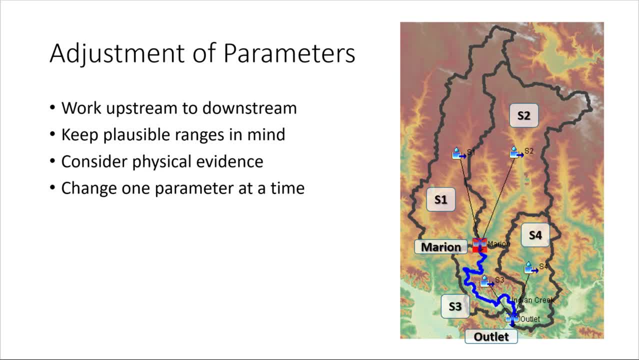 When calibrating for the outlet junction, you should leave everything above the Marion Junction alone once the performance at Marion is satisfied. When calibrating, keep in mind what ranges for a parameter are reasonable. If you are pushing against the boundary of reasonable values in your calibration. 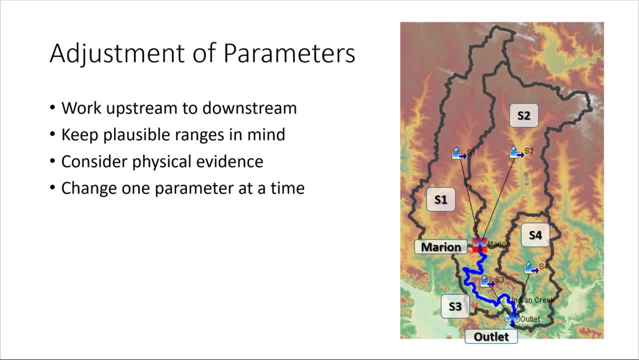 perhaps you need to be adjusting something else to bring that parameter back into range. Consider why the model is behaving the way it is and consider the physical explanation for hydrologic behavior. Look at physical information to explain why the model behaves differently in different parts of the watershed. 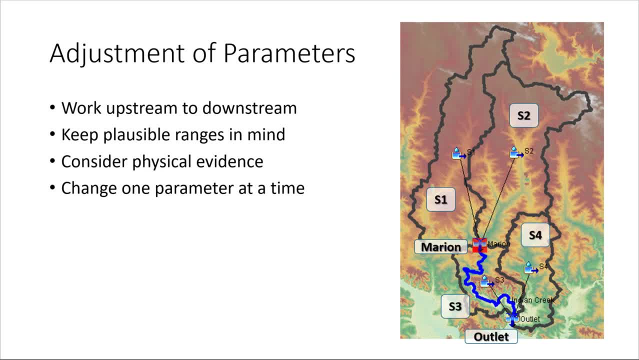 For example, parts of the watershed with poorly drained soils should probably have a lower infiltration rate than areas with well-drained soils. To really get a sense of the magnitude and direction of change on model performance you get by changing a parameter, change one parameter at a time and re-run the model. 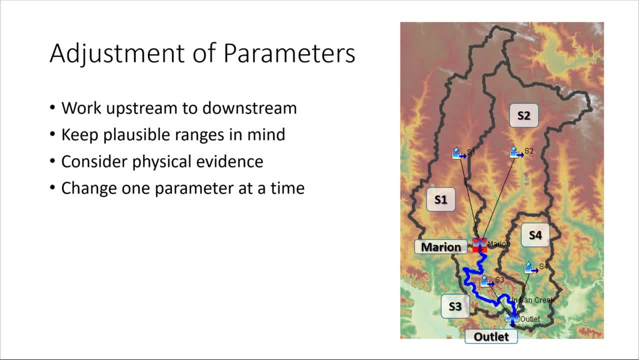 Then, when you feel good about the model performance in one aspect, such as timing or volume, you can move on to another parameter to change that parameter. This isolates the effects of the parameters and gives you feedback on how sensitive the model performance is to that parameter. 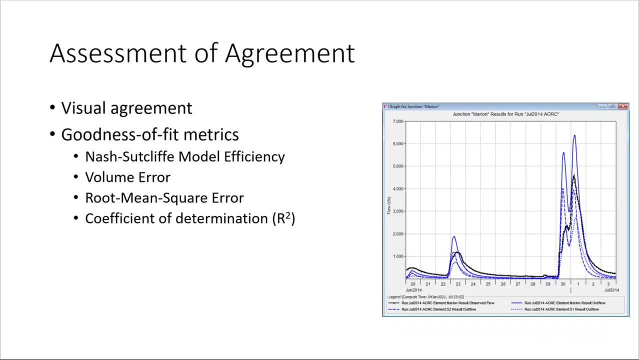 In order to understand the effects of the parameters, in order to assess model agreement, you need to be able to compare the model output to observed data. In HEC-HMS, observed data is shown in black, with the simulated results in blue. Visual agreement is the first step. 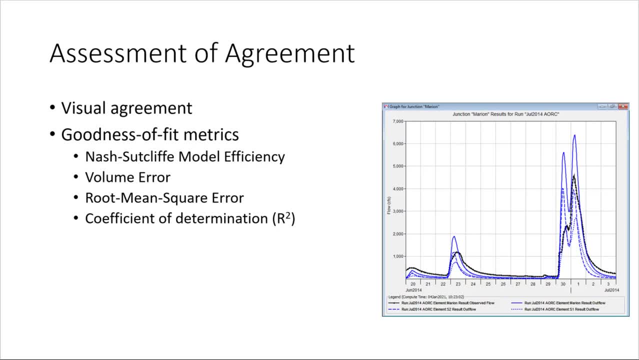 It lets you qualitatively assess things like timing, volume, hydrograph shape and so on. When you're calibrating, you can get a long ways just by using a visual comparison. Eventually, you get to a point where it's hard to know objectively. 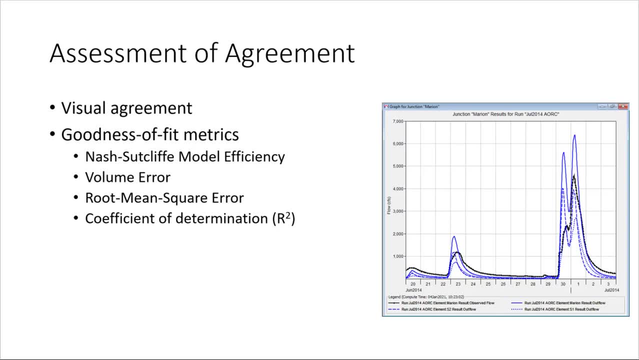 whether one parameter set is better than another, and goodness-of-fit metrics can help. They can also give you an idea of how good your agreement is. numerically, Four common goodness-of-fit metrics are shown here. There are guidelines for what values of these goodness-of-fit metrics. 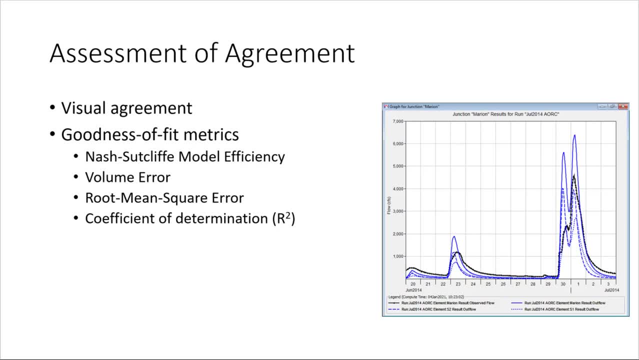 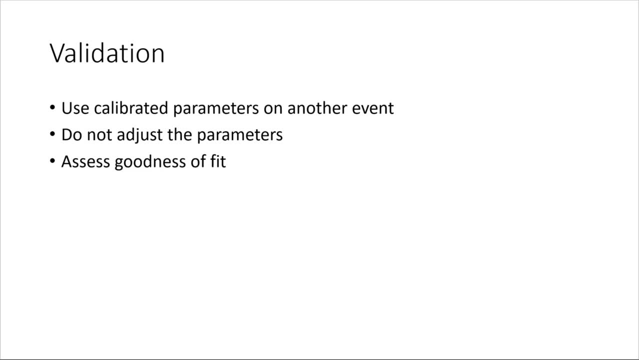 describe good agreement between the model and observed data. These concepts will be discussed in another video. Validation is an extremely important and often overlooked step. It assures that you have not over-fit your parameters to a single event and that the model has predictive power outside of just the calibration period. 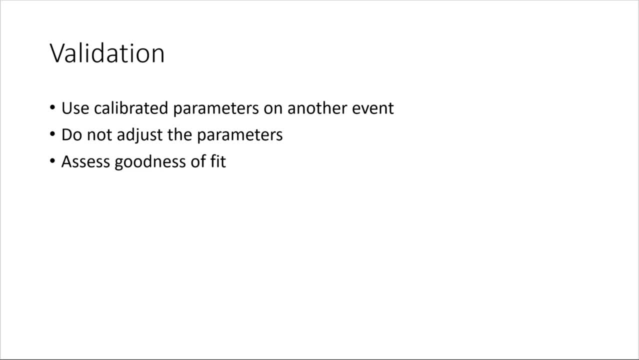 A mistake often made is that a modeler will start to alter parameters during the validation process, but then the independent assessment of the model performance is ruined. The only parameters that might change in a situation like this are initial conditions, for example, initial deficit, initial base flow and so on.